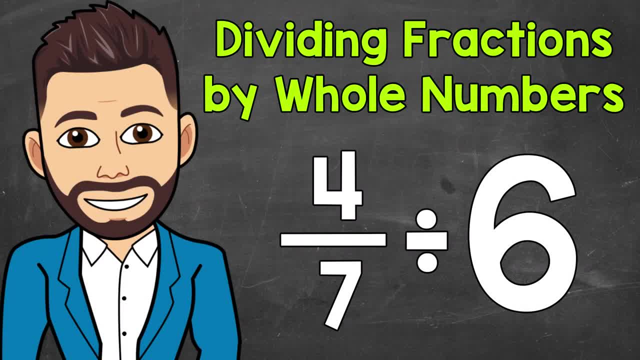 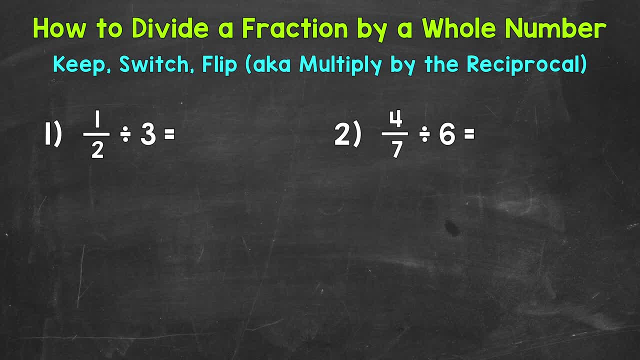 Welcome to Math with Mr J. In this video, I'm going to cover how to divide a fraction by a whole number. Now, when working with fractions and division, we need to remember three steps: Keep, switch, flip. We can also think: multiply by the reciprocal. 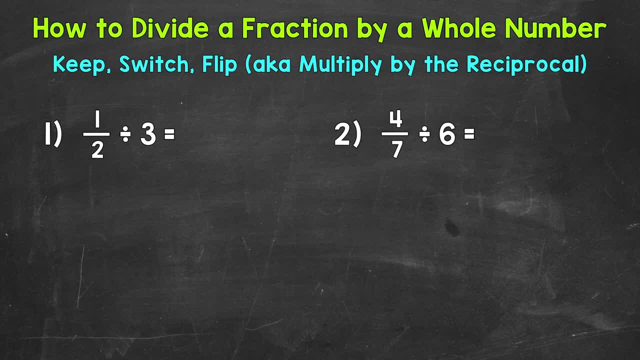 When we flip a fraction, that's called the reciprocal. So this means we are going to use multiplication to solve these. This actually makes the process simpler. Now, how and why this works is a topic for another video. I'll drop that link down in the description. 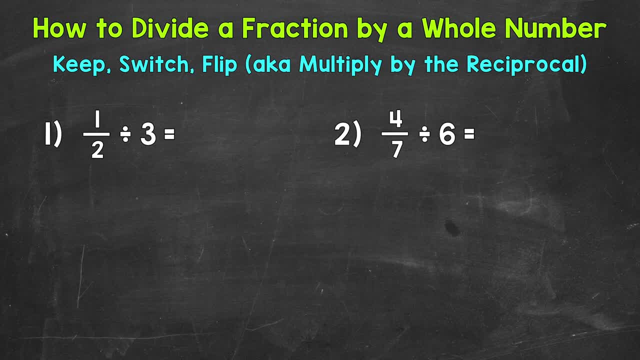 Let's jump into number one, where we have one half divided by three. So we are taking one half and dividing it into three equal groups or parts. Let's rewrite the problem using keep switch flip in order to solve this. So always keep. 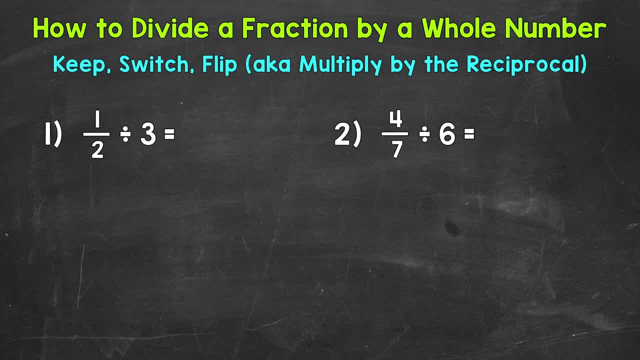 The first fraction or number. So let's rewrite the problem. So one half we are going to keep. Then we switch to the opposite or inverse of division, which is multiplication. And since we switched to multiplication, we need to flip the second number or fraction. 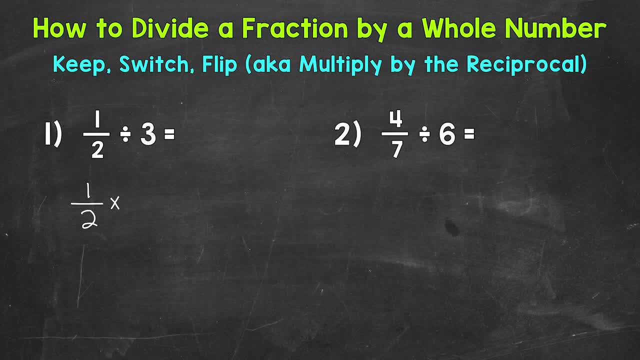 In the case of number one, we have a whole three here. So how do we flip this? Well, let's put that whole number over one. That way we have a numerator and a denominator That does not change the value of the problem. 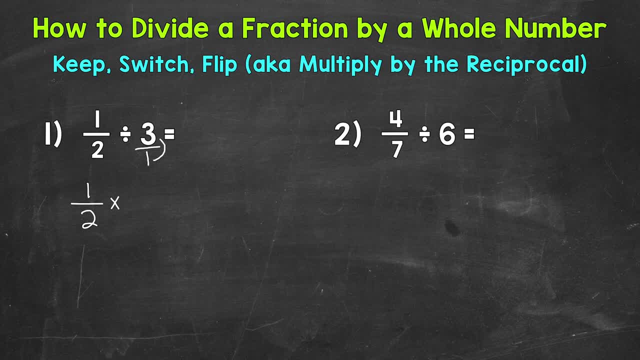 That still has a value of three. So now we can flip. So the one is going to go up to the top and be our numerator And the three is going to be the denominator. So we flipped that second number. Once we get to this point we have a multiplying fractions problem. 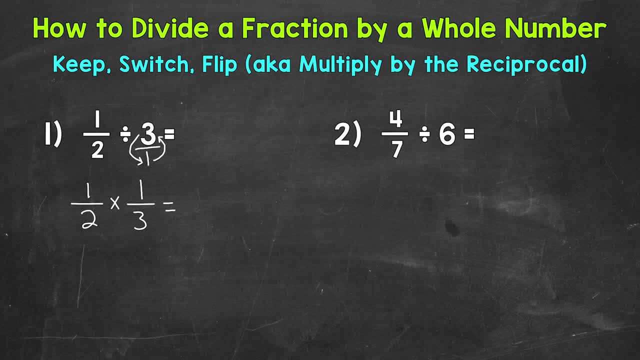 So we can multiply straight across: One times one is one And two times three is six. So one sixth is our final answer. Always check to see if you can simplify. One sixth is in simplest form. So we are done. One half divided by three equals one sixth.